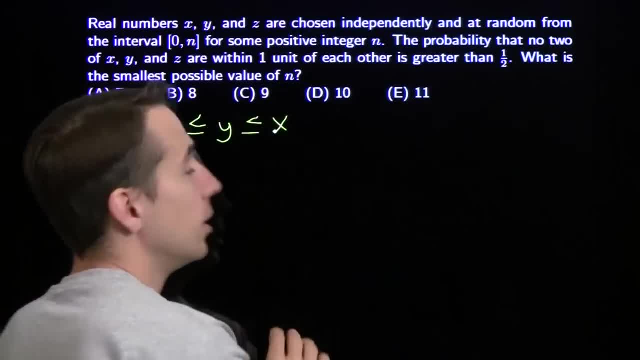 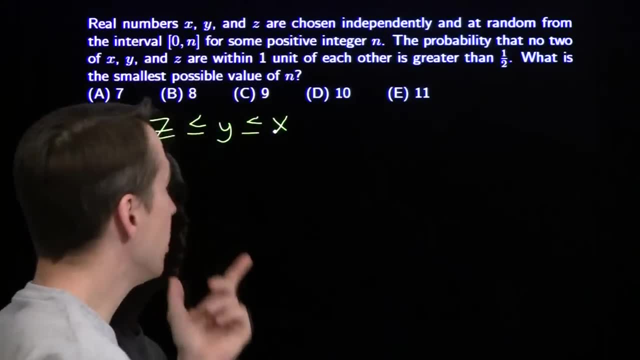 less than or equal to y is less than or equal to x. We're just going to look at this case Now. there are six possibilities for the order, because there's three factorial ways to order these three variables. We're just going to look at this one Now. we expect that to just 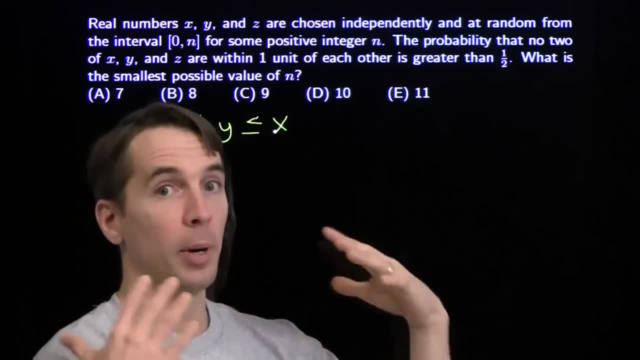 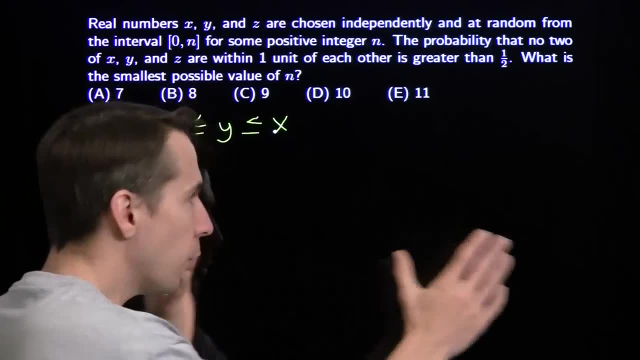 cover n cubed over 6.. That would be the volume of our possible space, space because this is. we expect this to be 1, sixth of all possibilities. So, as we proceed, whatever we come up with for our volume of the possible shape, with 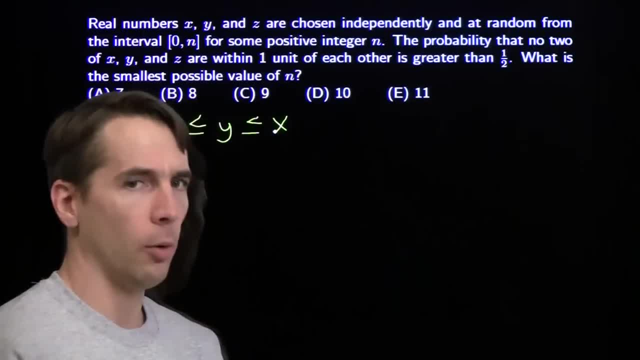 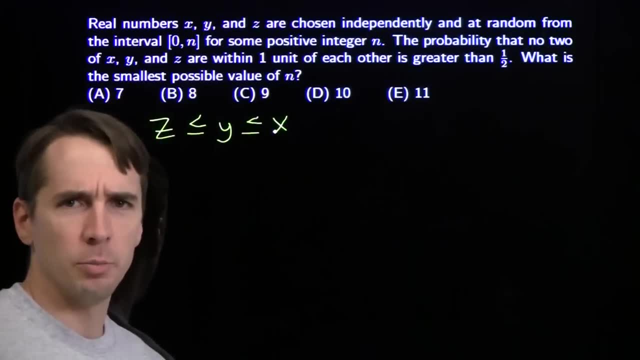 this restriction. it better come out to be n cubed over 6, or we've messed up Now to think about: well, how are we going to do this now? well, we're going to start drawing some pictures, And it's hard for me to think in three dimensions once we start putting in a bunch of restrictions. 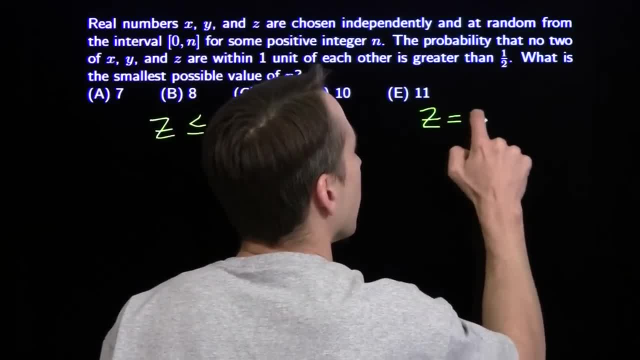 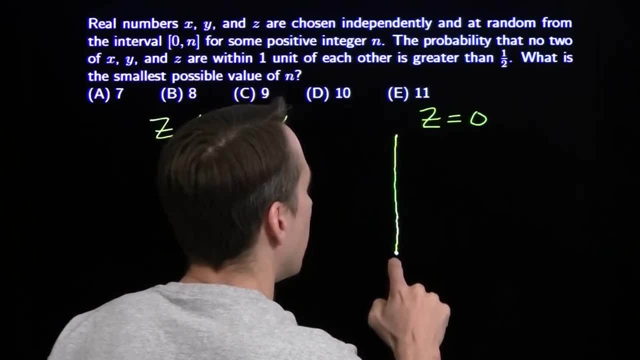 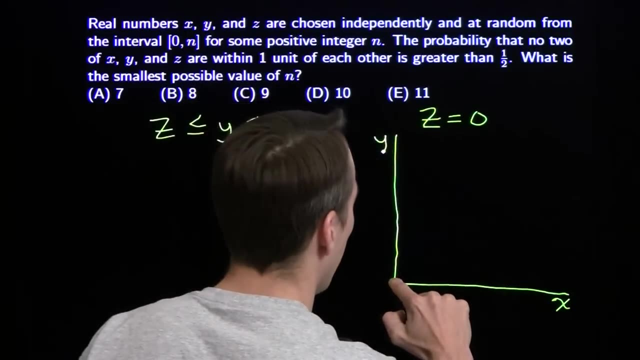 So I'm going to start off just by thinking about one possibility. Let's look at z equals 0.. What happens if z is 0?? Well then I'm going to draw x and y, and I need x to be greater than or equal to y. 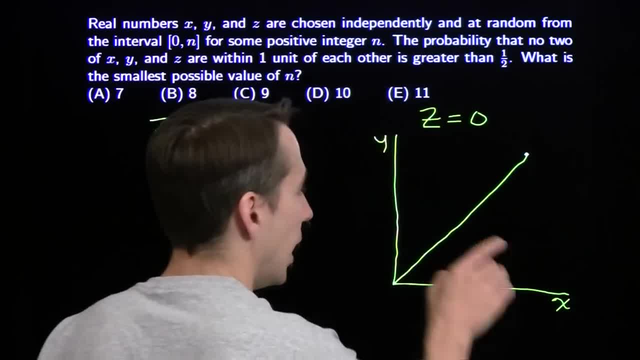 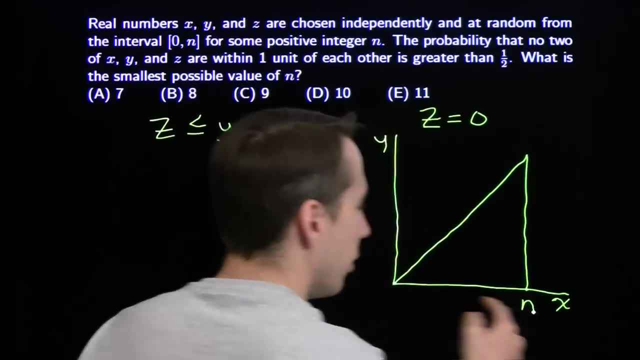 So I can start off by going like this: and x is greater than y, so I only want the stuff over there and let's go ahead and limit it at n. We'll call this n, So we can't go beyond there, because then x will be greater than n. 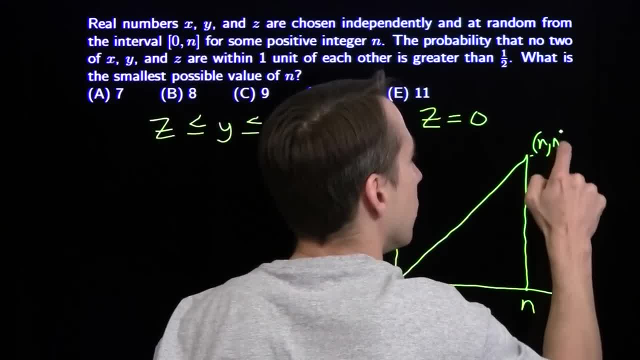 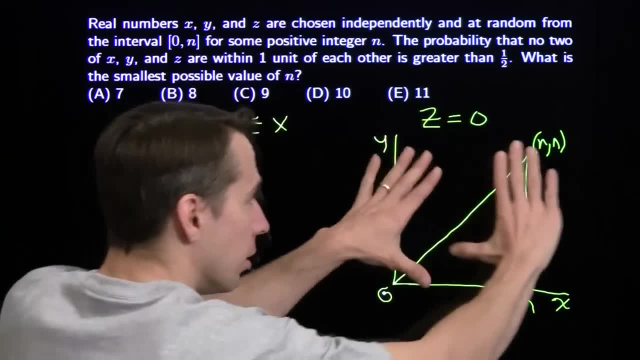 This point up here. this is nn And this is the origin. This is 0.. Now, at first it looks like, well, x and y can be anything in here. all right, So this is our possible space. if we want x is greater than or equal to y and that y 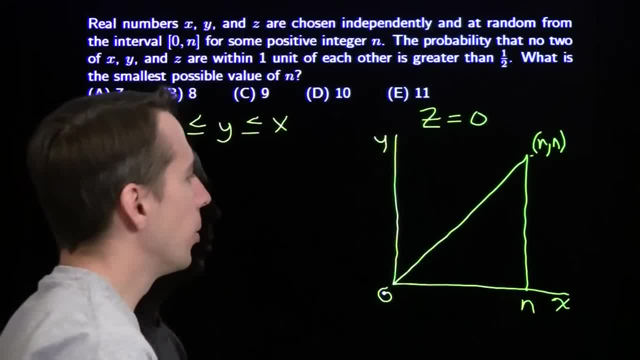 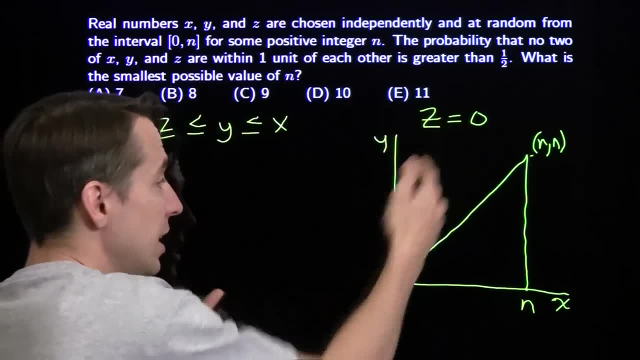 is greater than or equal to 0, greater than or equal to z, and z is 0.. So now we need to think about our successful outcomes. No two of them are within one of each other. Well now, z is 0.. 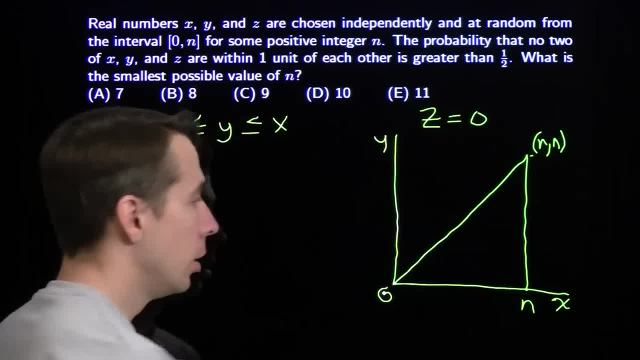 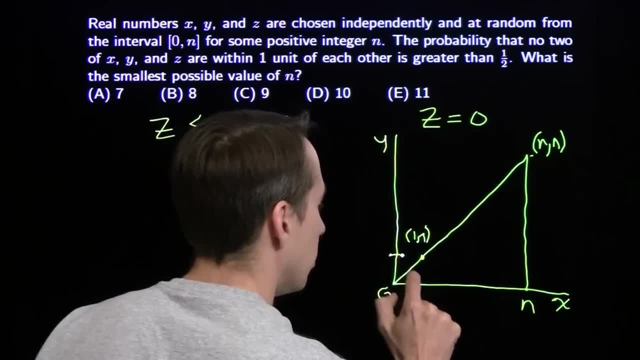 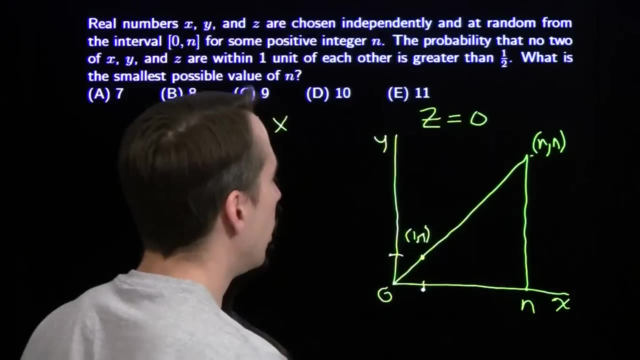 And that means x and y have to be at least 1.. So we can start off just by thinking about this point here: 1, 1.. We'll call that 1, 1. And we know that x and y- neither of them- can be less than 1, so we can't be down here. 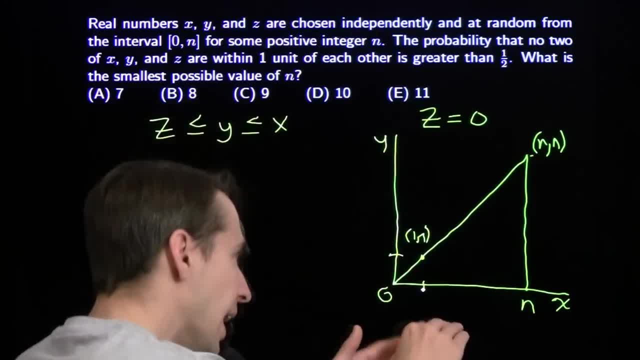 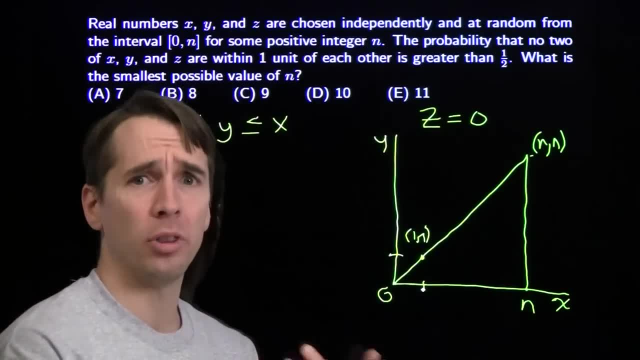 y can't be less than 1, so we can't be down here either. y has to be at least 1, so we've got to be up here somewhere. And then we also know that x has to be at least 1 more than y. 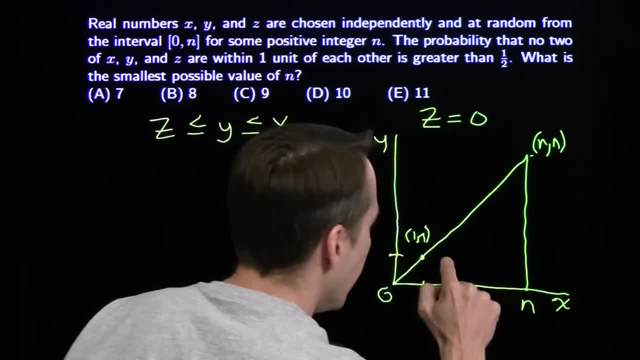 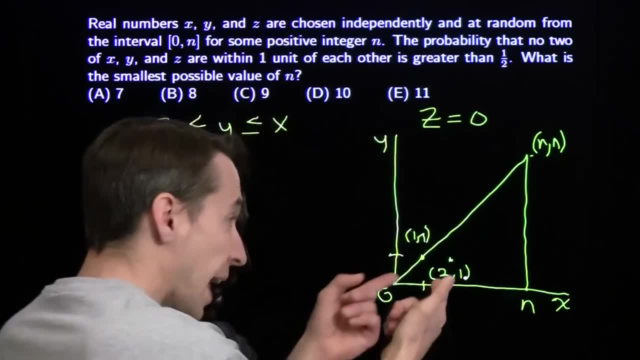 So that's a further restriction. That means that wherever y is, you know, say we started right here. call this point 2, 1.. That's okay. x is 2.. y is 1.. z is 0.. 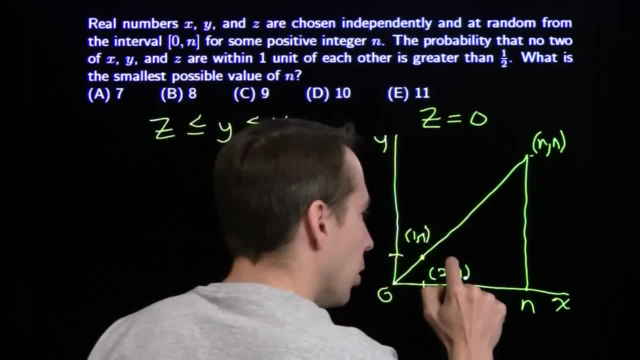 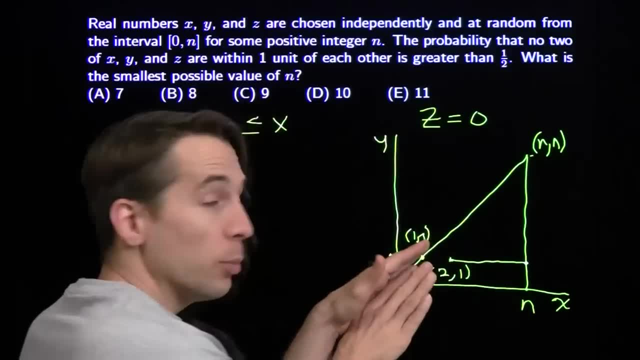 That's all fine. Now, from here, x can be anything larger than this. So everything on this line, this is just fine. But then as we increase y, we need to increase x as well. So if y is say 2., then x has to be at least 1.. 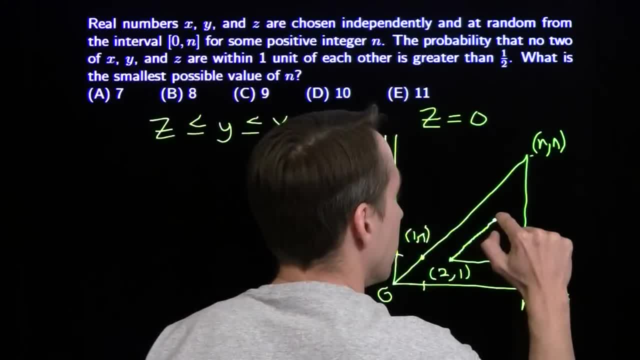 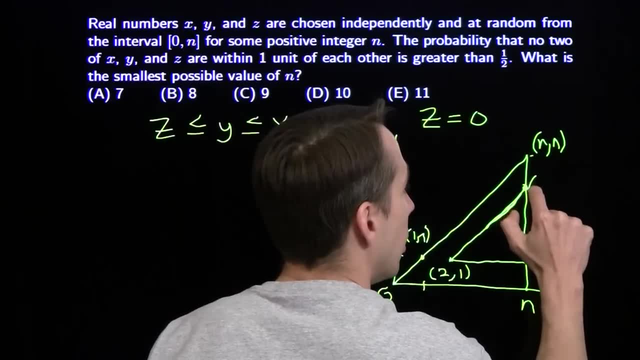 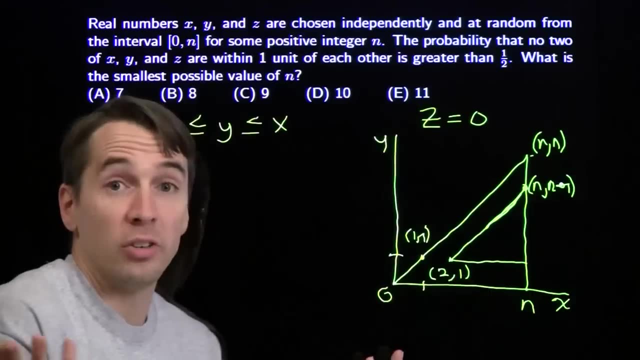 x has to be at least 3.. We're moving along this line. We get all the way up to here, where x is n and y is n minus 1.. y can't ever get larger than n minus 1, because once y is larger than n minus 1, there's nothing. 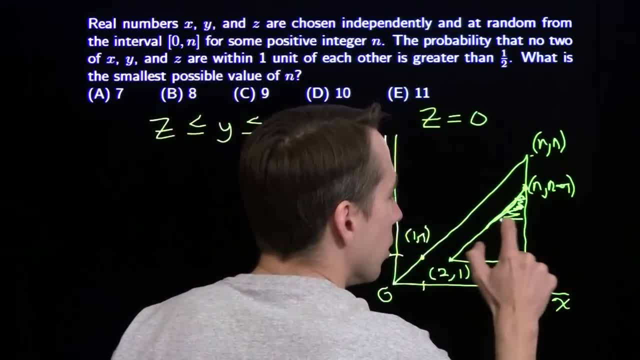 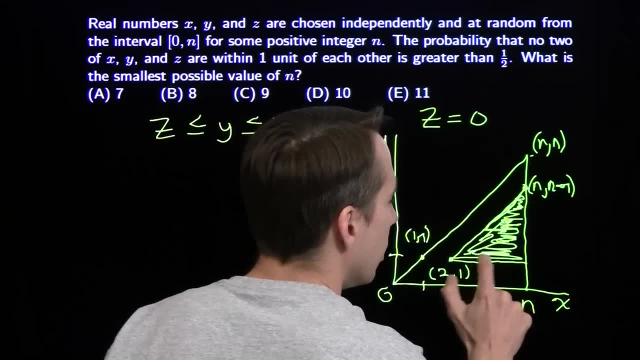 that x can be, But we can be anywhere in here and we're just fine. Everywhere in here, x is at least 1 more than y, And we're just fine. We're just fine, And y is at least 1 more than z. 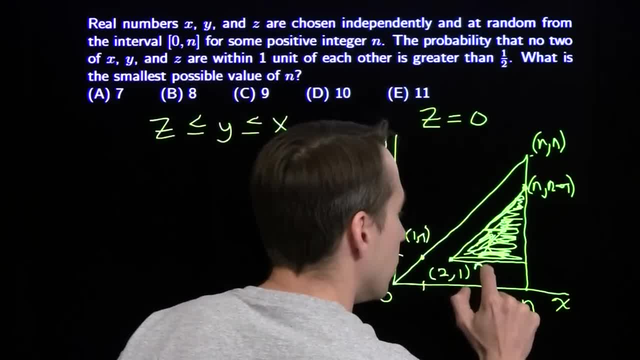 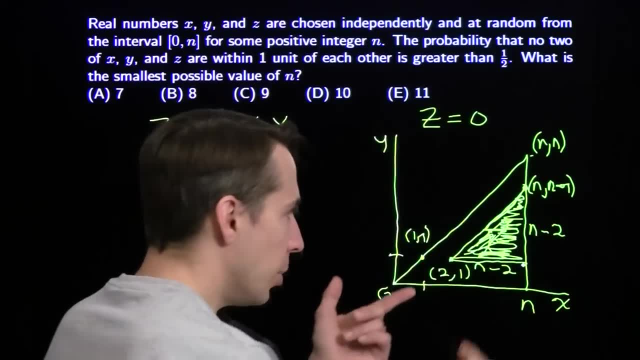 So everything in here is just fine. In this triangle its leg lengths are n minus 2, because this right here is at y equals 1.. This is at y equals n minus 1.. So this is an n minus 2 by n minus 2 triangle. 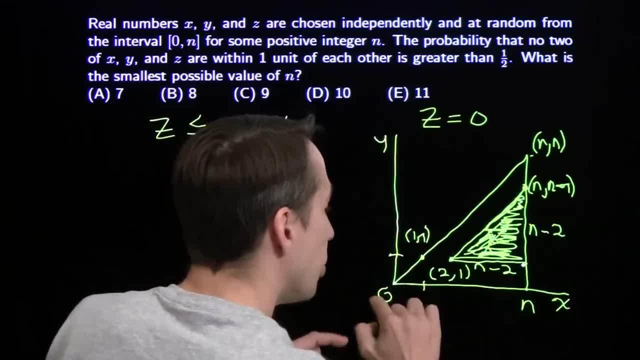 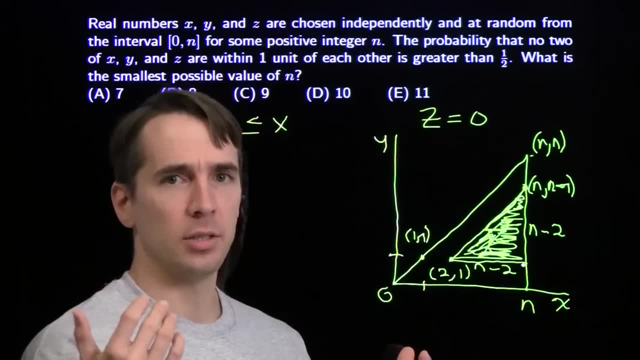 This is a successful region. These points are okay. This is our possible region. It's the same shape triangle, but it's n by n. Now let's think about what happens. as z increases, Say, we move z up to 1.. 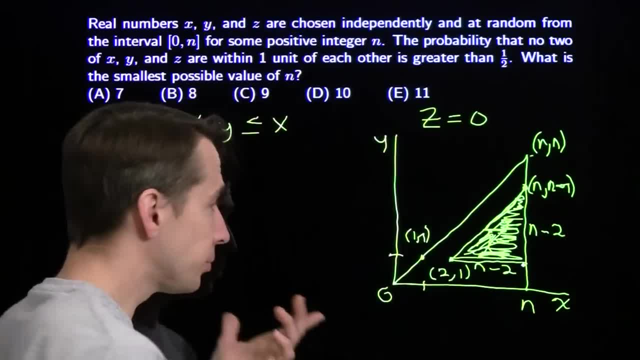 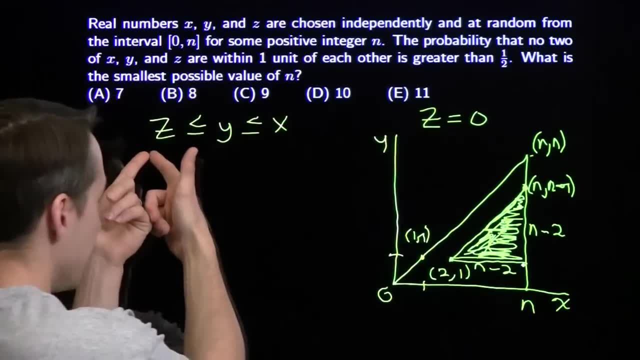 Well, now, now our possible region, our possible region if z is 1,. x and y both have to be greater than 1, because we're going to have this: z is less than or equal to y is less than or equal to x, and we still need x to be greater than or equal to y. 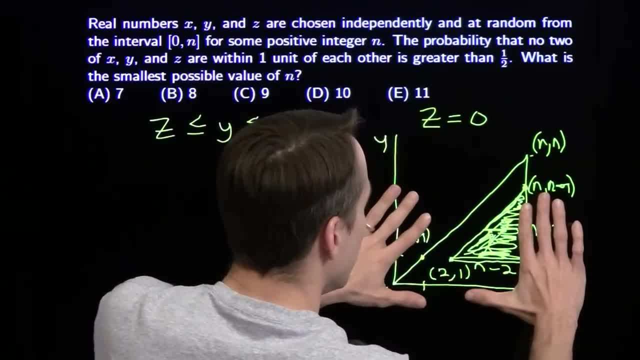 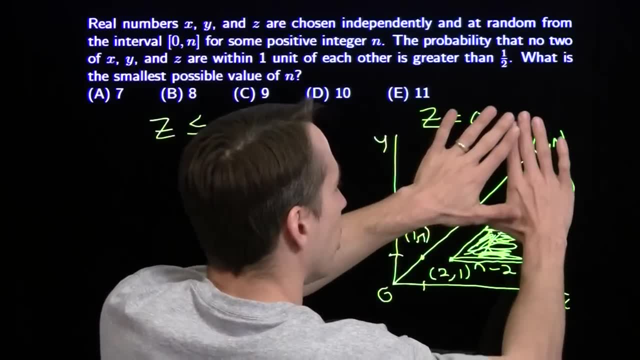 So instead of this whole triangle here, when z is 1, we'll move up to this triangle here. The triangle gets smaller and as we move z higher- z equals 2, it gets smaller, smaller and smaller. It comes all the way up to the point n, n, n, when all three are n. 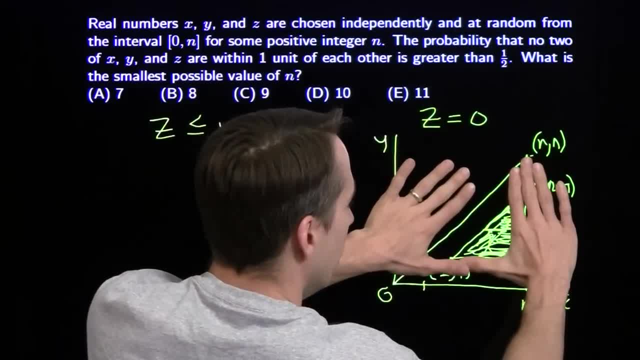 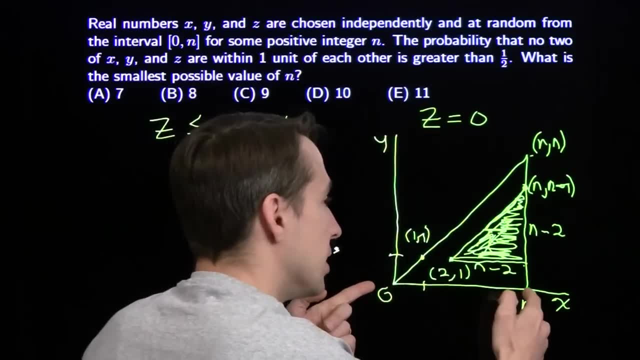 So here it is. when z is 0.. When z is 1,, well, we can't have x or y be 1 or smaller anymore, and we get smaller and smaller and smaller. We're forming a pyramid. The base of this pyramid is an n by n triangle, isosceles right triangle that has area n squared. 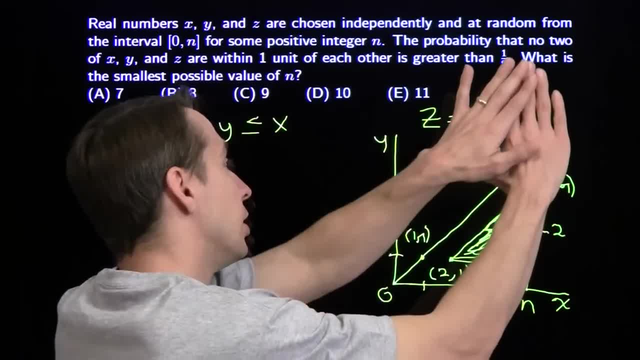 over 2.. The height of the pyramid as we come out from this is going to be n, because we're going to go all the way up to n by n, by n. So I have a pyramid. The base area is n, n squared over 2.. 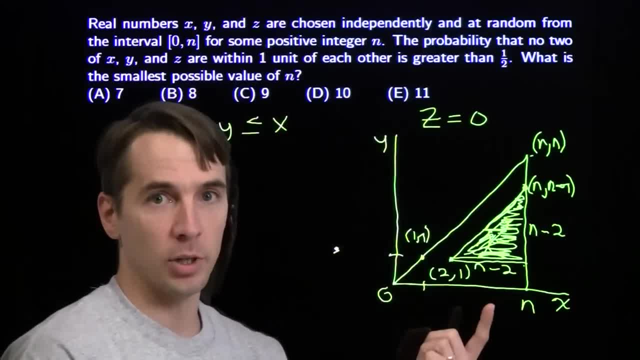 The height is n, The volume comes out to be n times n squared over 2.. That's n cubed over 2.. And then we divide by 3, because it's a pyramid, We get n cubed over 6.. 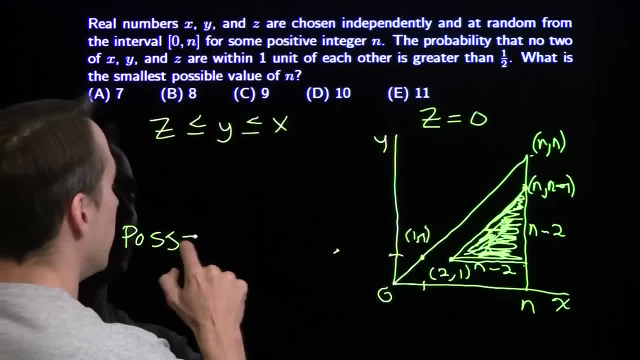 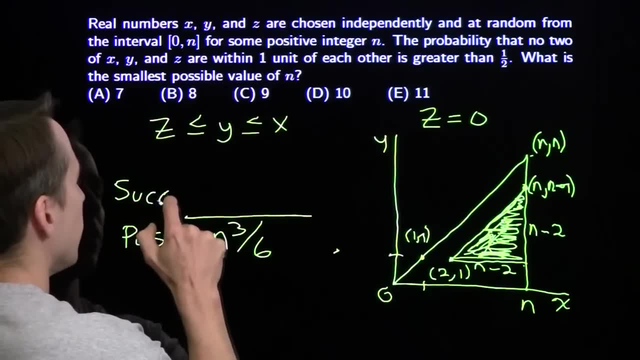 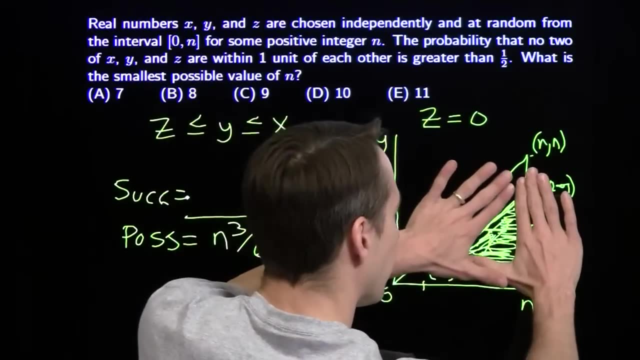 So there's our possible region. Our possible volume is n cubed over 6, as planned. What about our successful region? Our successful region is doing the same thing. It starts off as this: n minus 2 by n minus 2 little triangle. 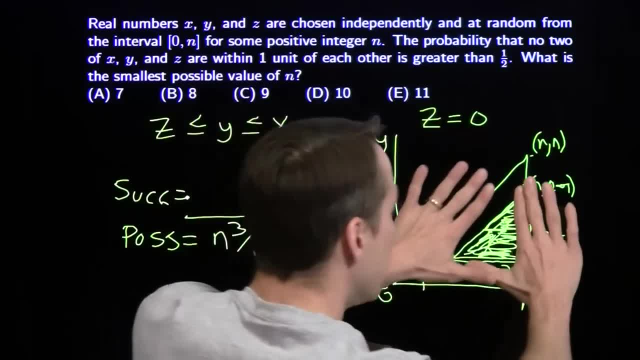 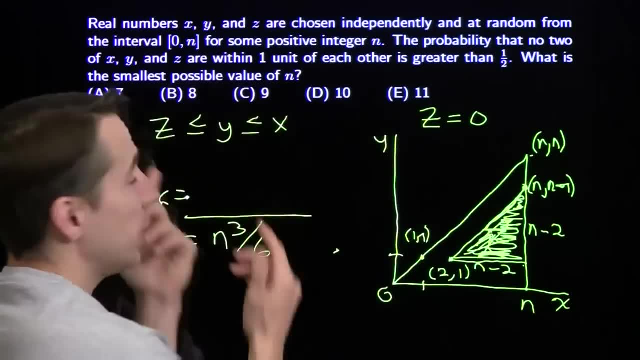 And then when z goes up, When z goes up, say when z goes up to 1,, this triangle gets one unit smaller. It's a little bit smaller because now, if z is 1, and we need them all to be at least- 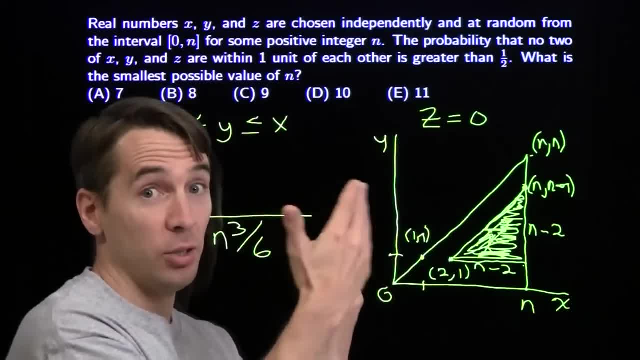 one apart. while z is 1, we can have y is 2 and x is 3.. We can't have 2 and 1 anymore. If z is 1,, we can have y is 2 and x is 3.. 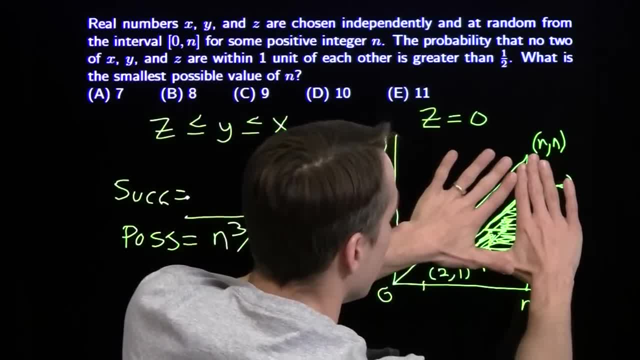 That moves this bottom line up 1 and over 1.. And this triangle also gets smaller and smaller and smaller. We're forming another pyramid, but this pyramid has the base is m squared over 2.. So we're going to have z squared over 2.. 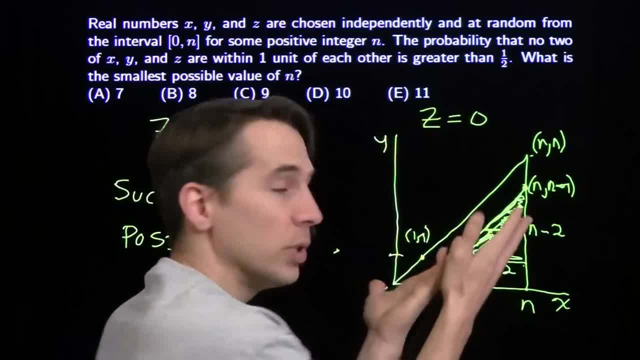 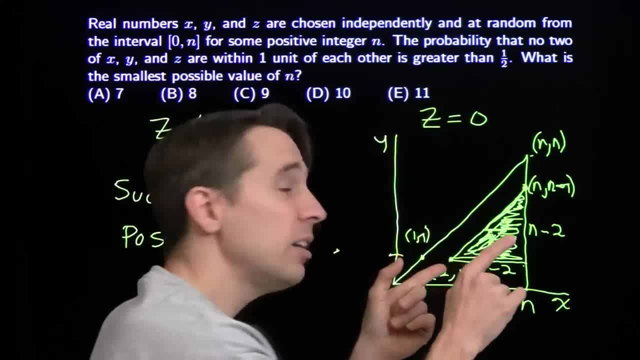 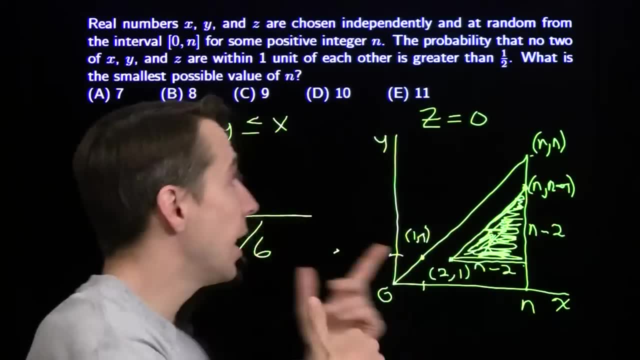 Its area is the square of n minus 2 divided by 2.. The height of this pyramid? this pyramid goes all the way up to n n minus 1, and then z would be n minus 2.. That's as high as you can get. 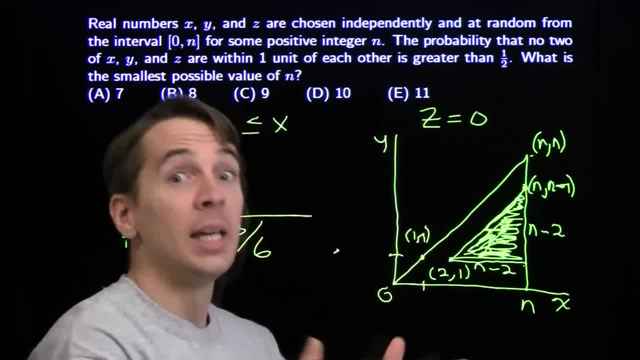 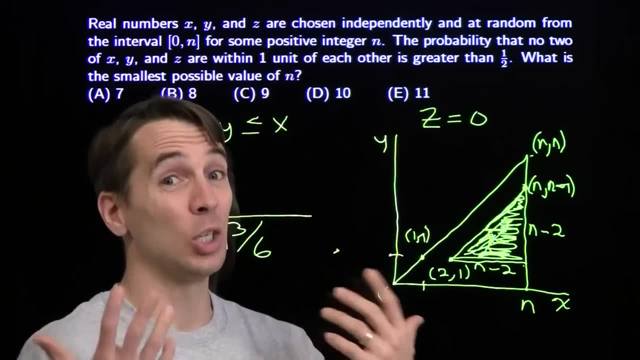 They all have to be at least one apart. So the height of this pyramid is n minus 2.. The base area is the square of n minus 2 divided by 2.. We multiply by the height, That gives us the cube of n minus 2 divided by 2.. 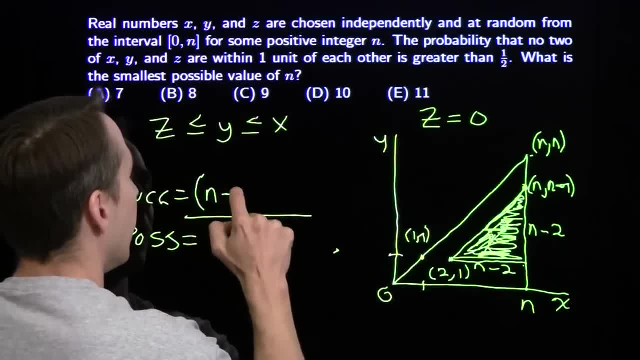 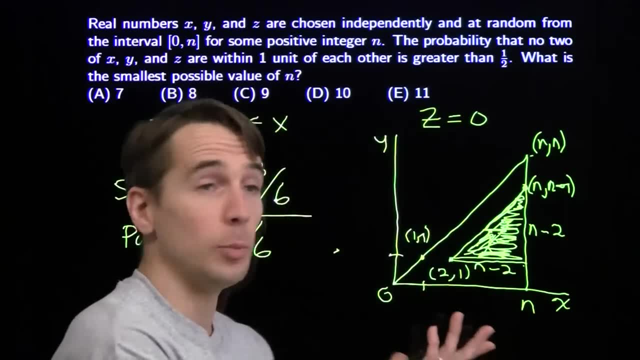 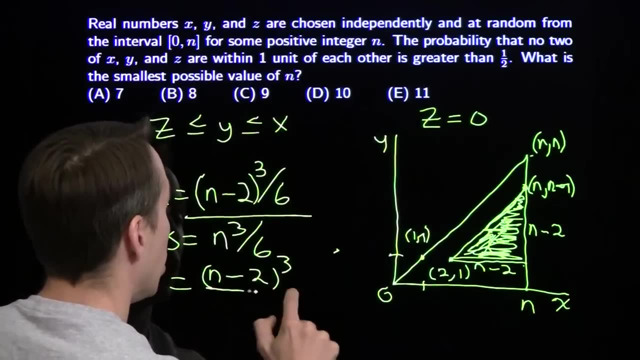 We have to divide by 3 again, because it's a pyramid. We have n minus 2 cubed over 6 is the volume of that region. This makes sense. These pyramids are similar, So the ratio of their volumes is just the cube of the ratio of their side lengths. 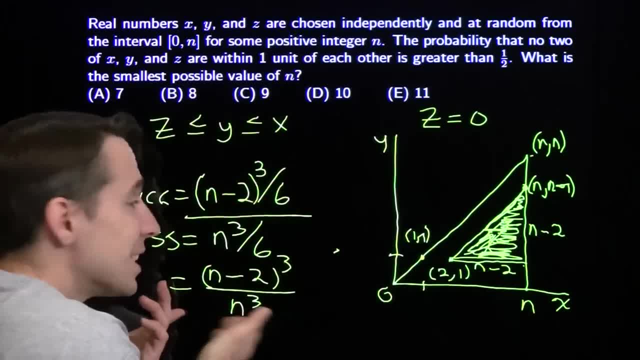 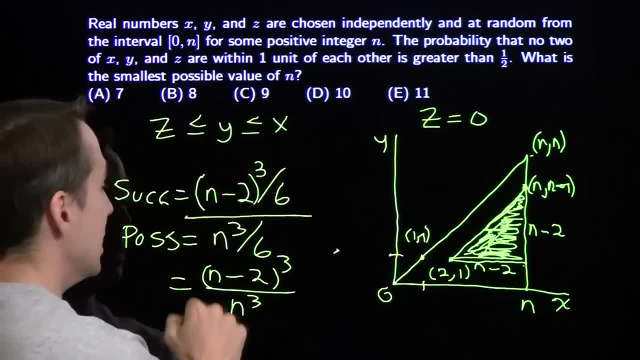 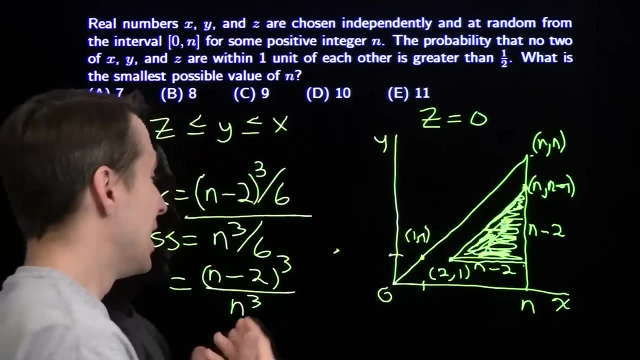 n minus 2 divided by n cubed. This is our probability and we need this to be greater than 1 half. Now we can just start sticking in some of this, Some of these choices. If we put in 9, we get 7 cubed over 9 cubed. 7 cubed is 343,. 9 cubed is 729,. 343 over 729,. 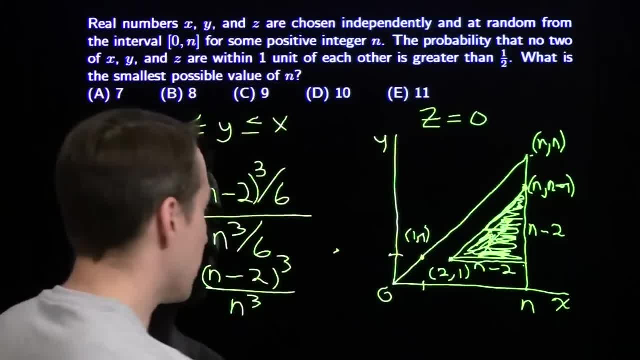 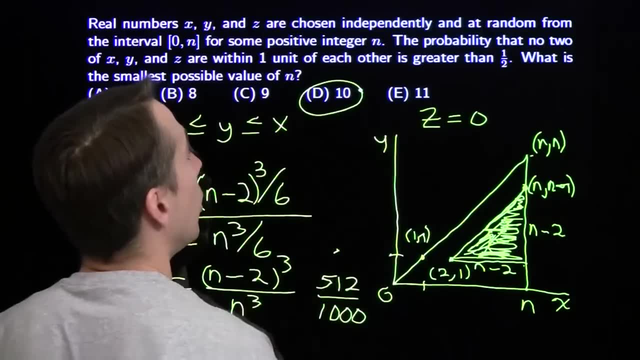 that's less than 1 half. If we put in 10, 10 minus 2 cubed, that's 512,. 10 cubed, of course, is 1,000.. So that's the first time that we will go over 1 half. 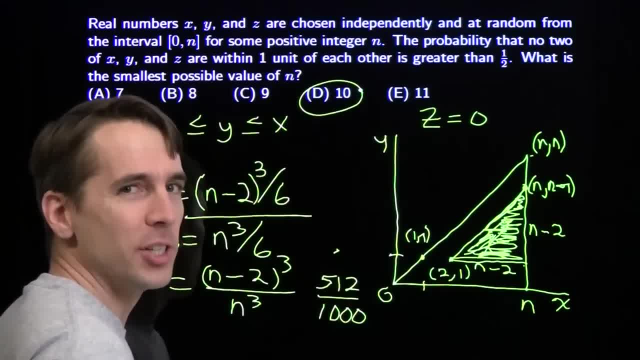 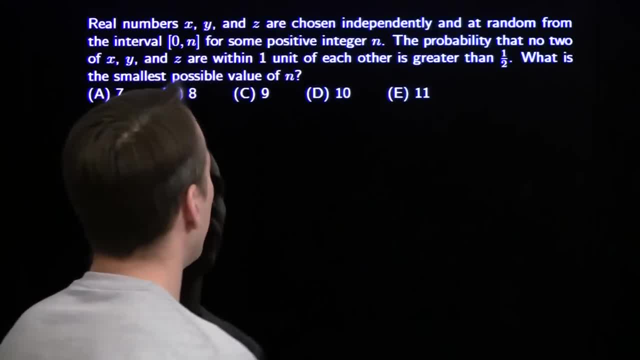 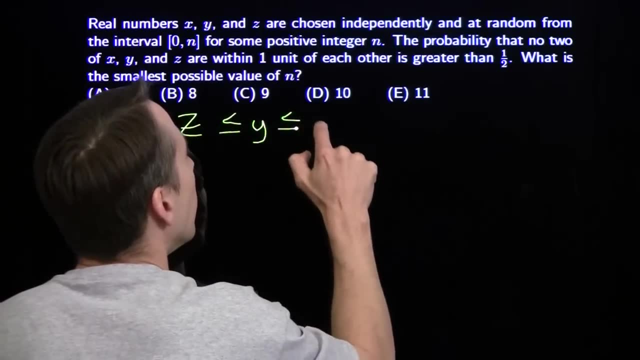 Now, you might find all this geometry a little fishy. Let's take another quick look at this problem, See if we can think about this entirely algebraically Now again. well, maybe just mostly algebraically. We'll still think about this a little bit algebraically, a little bit geometrically. 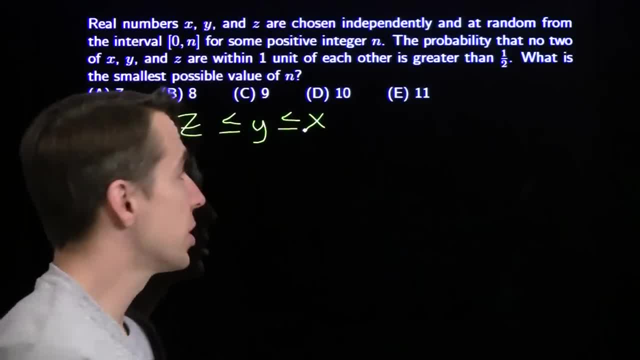 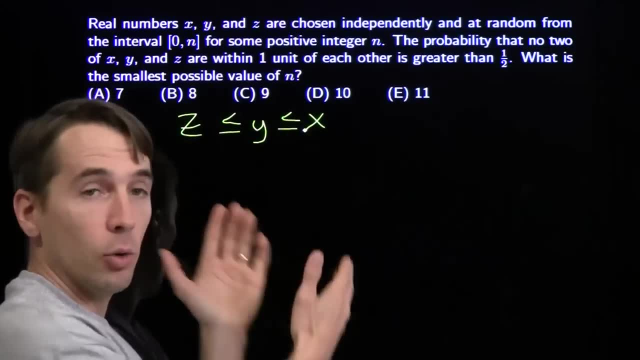 The space of possibilities for this is n cubed over 6, the volume of that space, As we explained before, n cubed- is the whole space, if we don't, if we let them be in any order. So if we impose an order like this, there's six possible orders. each of them there's 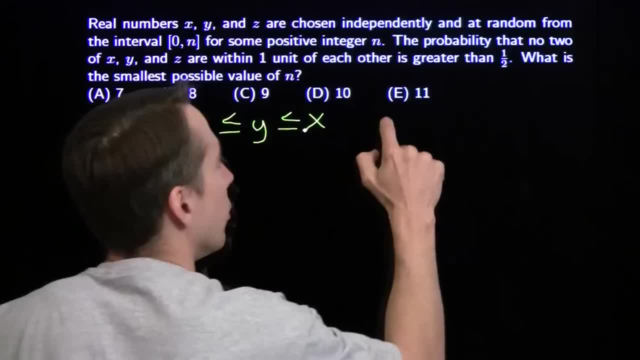 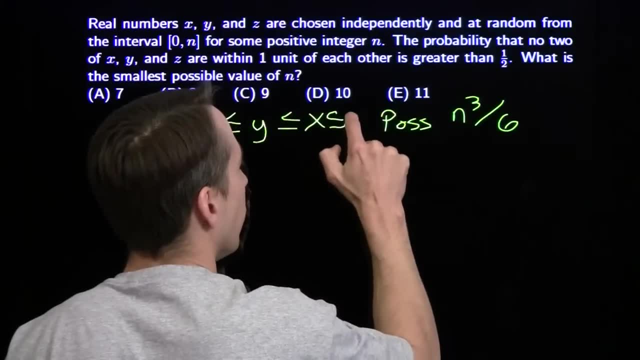 just symmetry. so each of them is 1 sixth of the whole space. so the possible space again is n cubed over 6, and the key here also is that this is less than or equal to n. Of course this is greater than or equal to 0.. 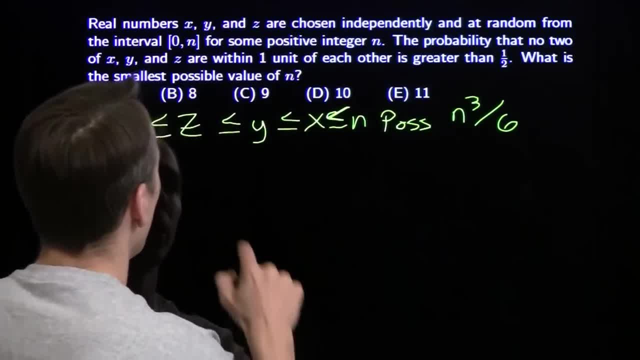 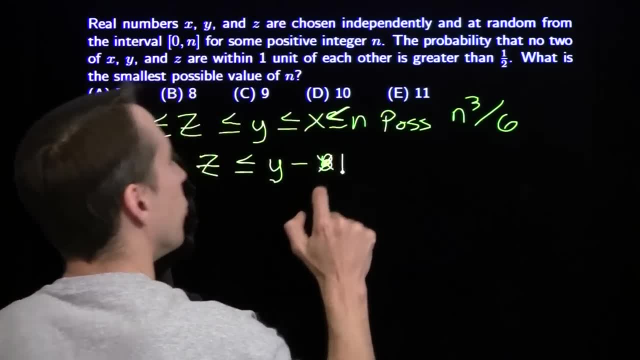 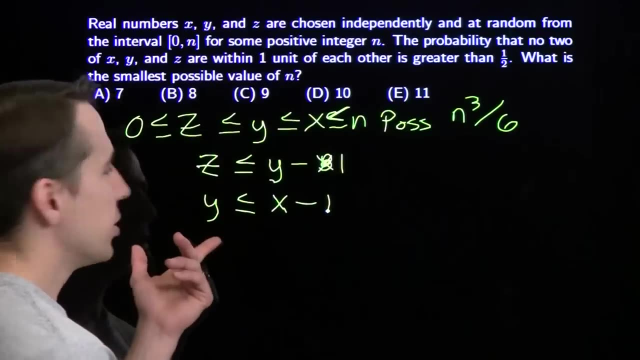 Now let's look at the restrictions we have here. All right, We have: z is less than or equal to y minus 1.. y minus 1.. And y is less than or equal to x minus 1.. These are hard restrictions to deal with. 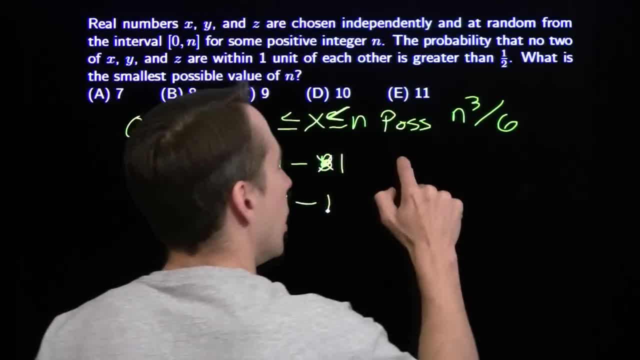 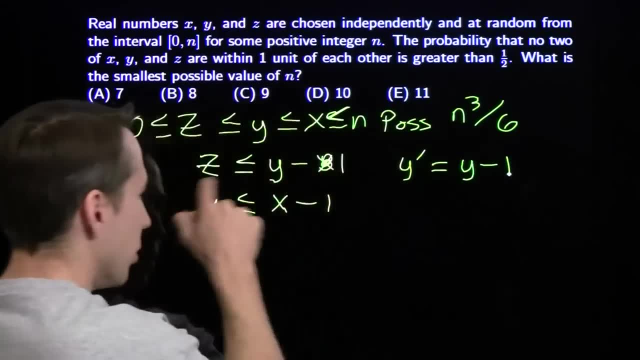 So we're going to make- we're going to make a little substitution. I want to turn this into a space I understand better. I'm going to put y prime equals y minus 1.. That's going to turn this inequality up here into: z is less than or equal to y prime. 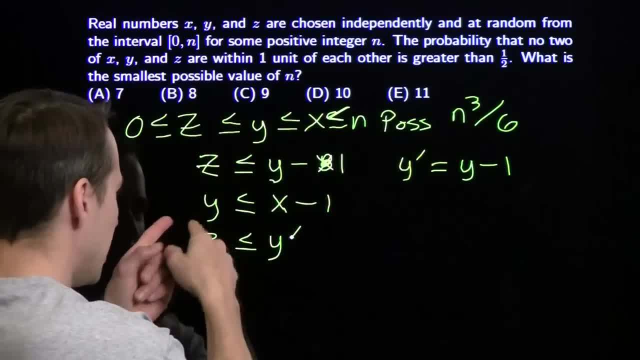 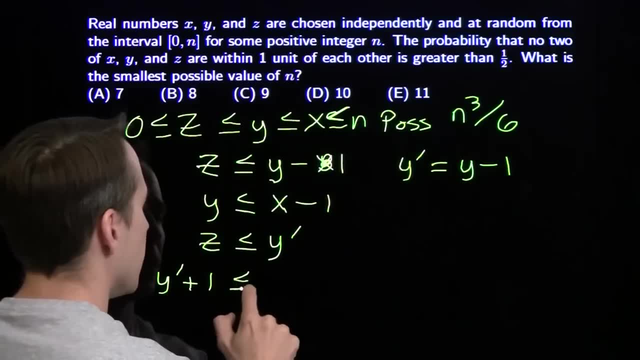 This is a lot easier to think about than that. Okay, And if I make the same substitution here, I'll have: y prime plus 1 is less than or equal to x minus 1, which means y prime is less than or equal to x minus 2.. 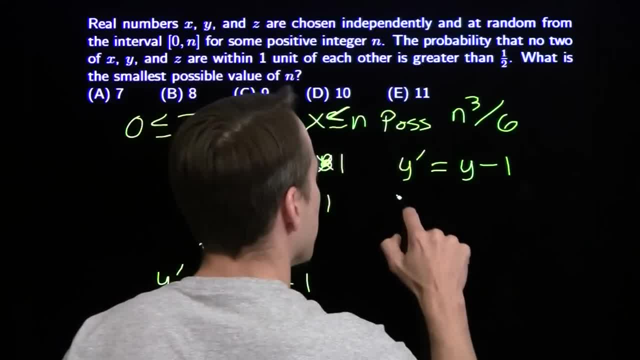 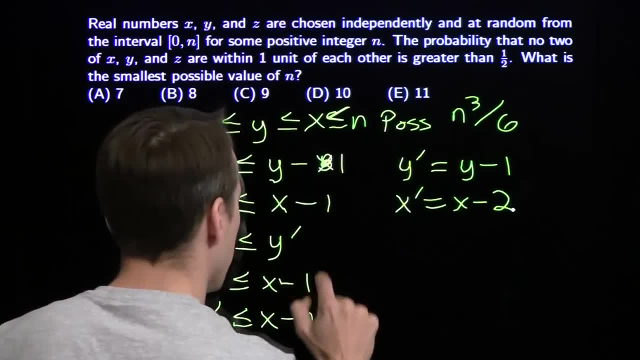 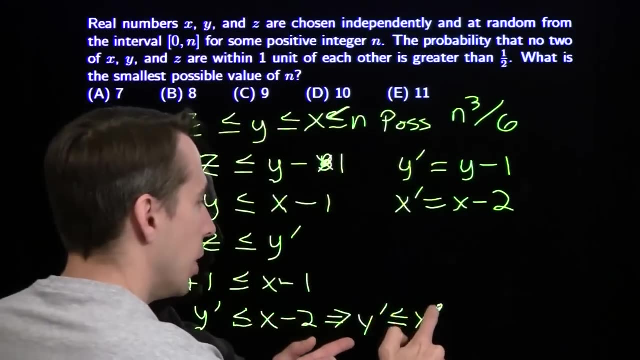 Let's make another substitution. I'm going to say x prime equals x minus 2, because that will turn this into: y prime is less than or equal to x prime, And that's a lot easier to think about as well. I can put these two together. nice and neat. 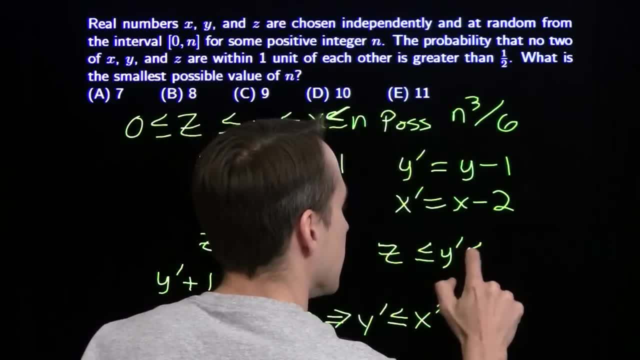 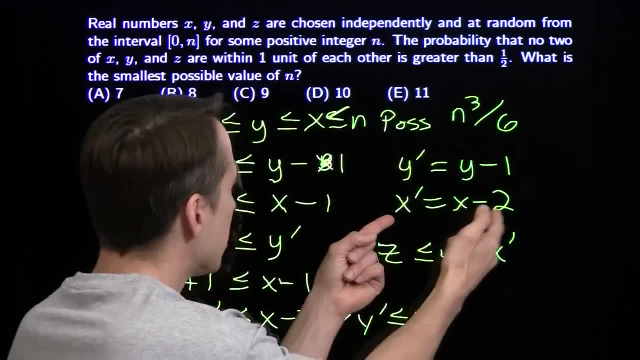 I've got: z is less than or equal to y, prime is less than or equal to x prime, And still, z just has to be greater than or equal to 0.. But what about x prime? Well, x prime is just x minus 2.. 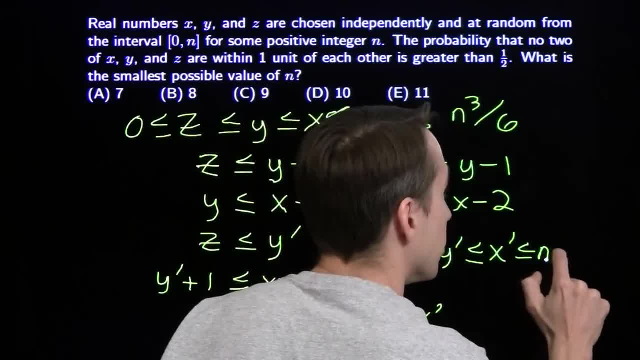 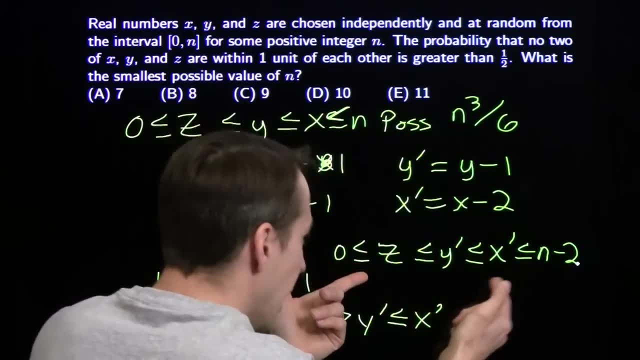 X has to be less than or equal to n, So this has to be less than or equal to n minus 2.. This is really easy to think about. We can think of this: We're just choosing x prime, y prime and z from 0 to n minus 2.. 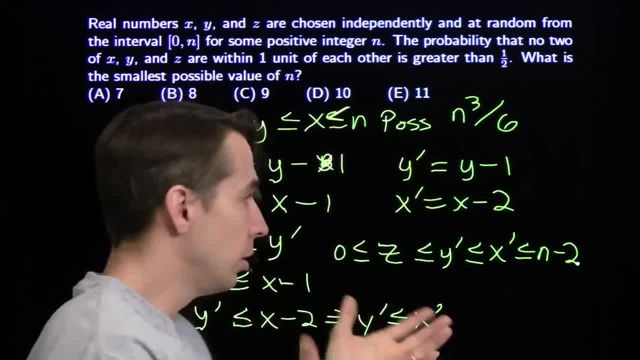 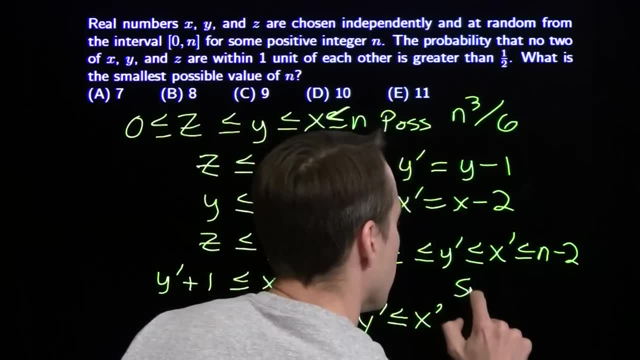 Now, if we did that without respect to order, if we didn't care about the order, there'd be a space of volume of n minus 2 cubed. Here we've got the order. There are six possible orders, as before. So that gives us our successful region. 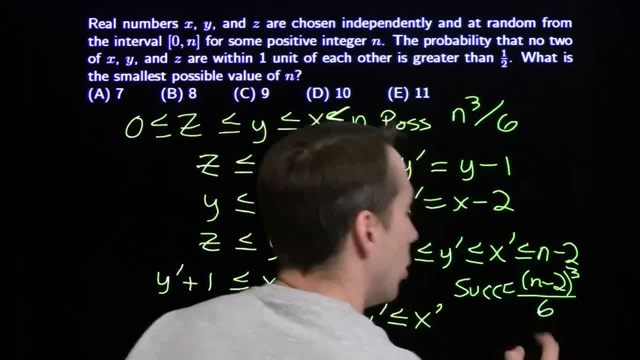 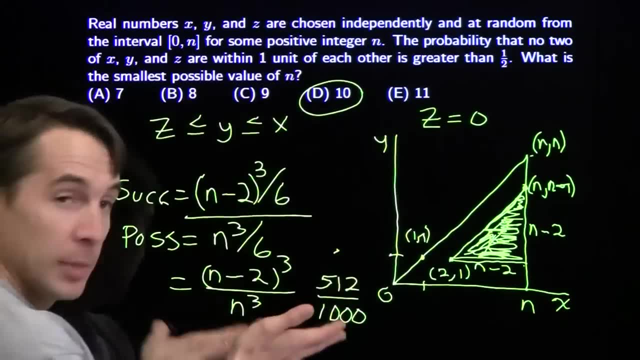 Its volume is n minus 2 cubed over 6.. This is a nice, more algebraic explanation for what we did before, when we come out with the same outcome- And we sure better come out with the same outcome. So we did the problem two different ways. 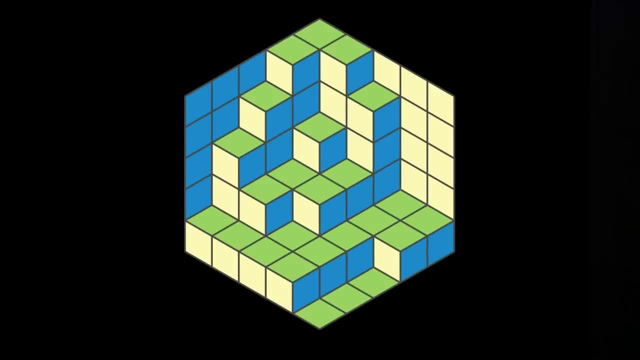 We got the same answer. We can be pretty confident we're right.